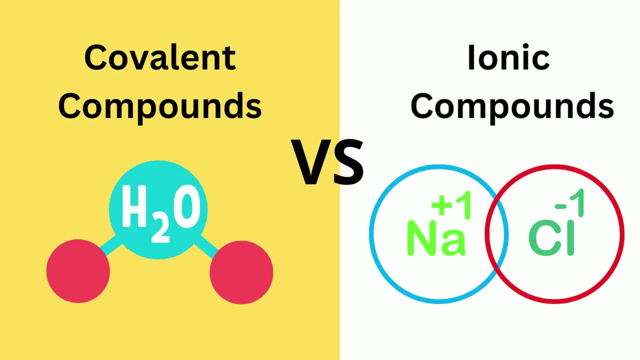 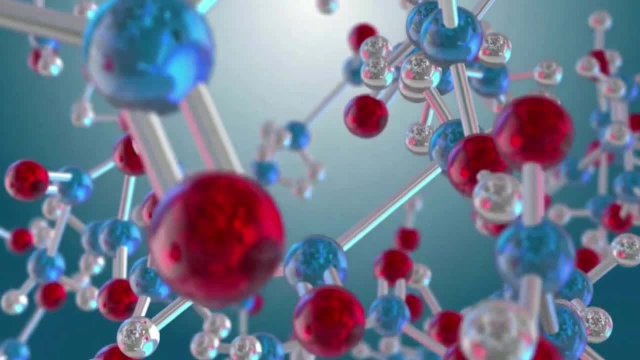 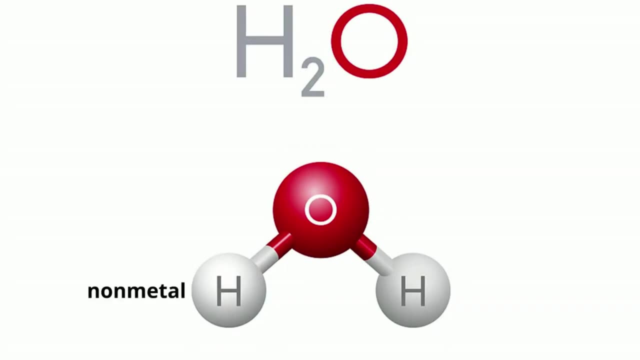 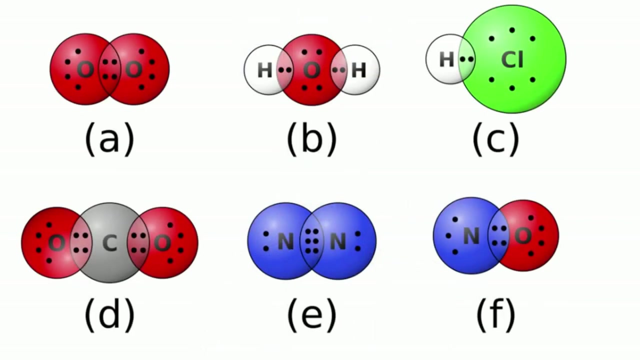 A molecule or compound is made when two or more atoms form a chemical bond that links them together. Covalent compounds generally result from two nonmetals reacting with each other. The elements form a compound by sharing electrons, resulting in an electrically neutral 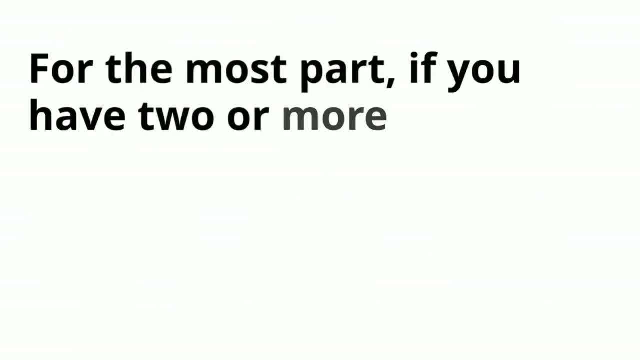 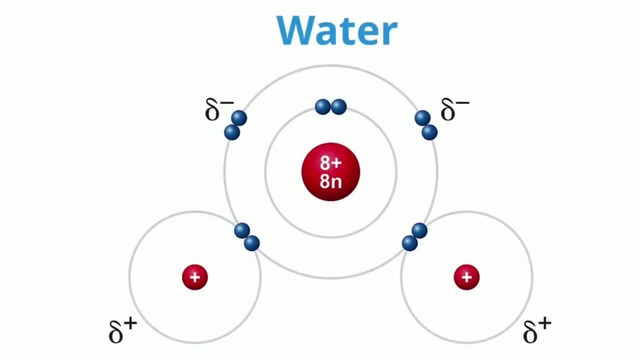 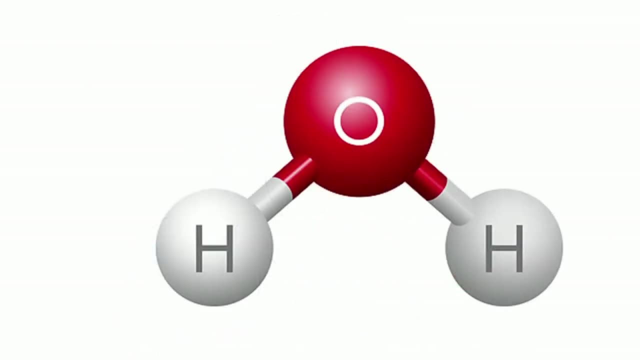 molecule. For the most part. if you have two or more nonmetals chemically combined it will be a covalent compound, For example in water. each hydrogen and oxygen share a pair of electrons to make a molecule of two hydrogen atoms, single, bonded to a single oxygen. 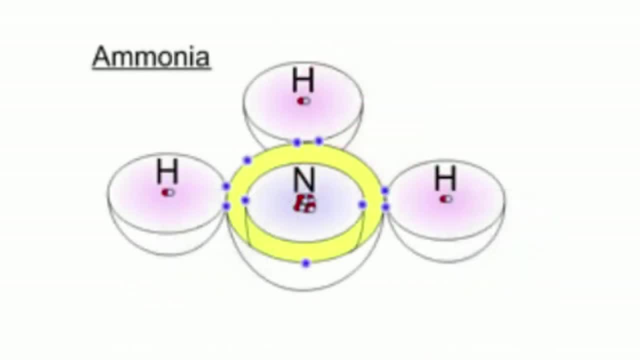 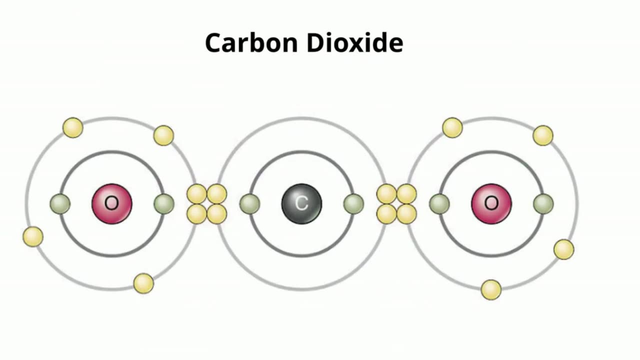 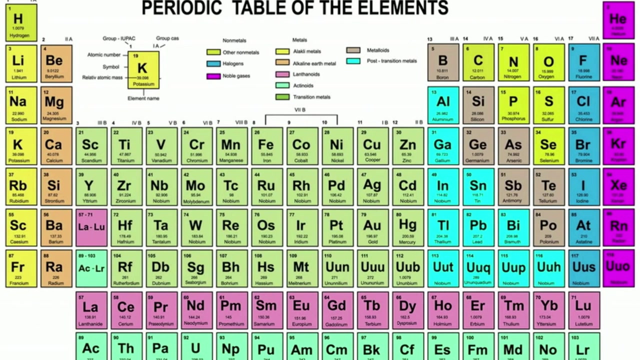 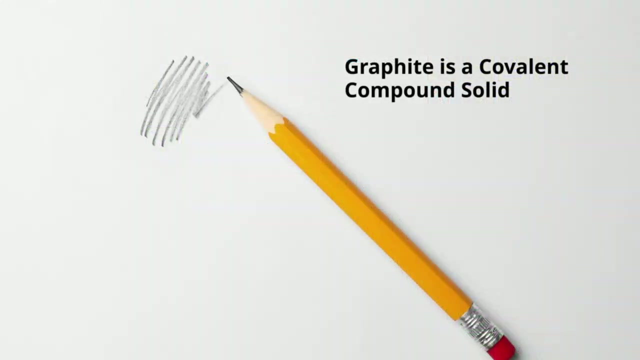 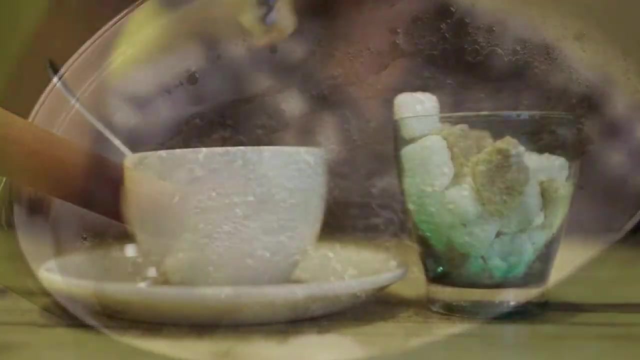 atom. Other examples include ammonia, chlorine and carbon dioxide. In general, covalent bonds occur between elements that are close together. on the periodic table, Solid covalent compounds tend to be soft. Covalent compounds have relatively low melting and boiling points. Some covalent compounds dissolve in water. 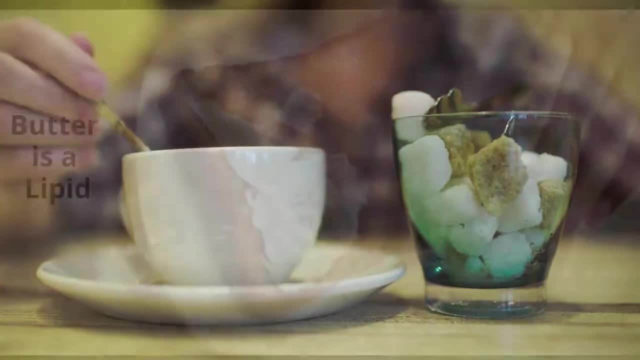 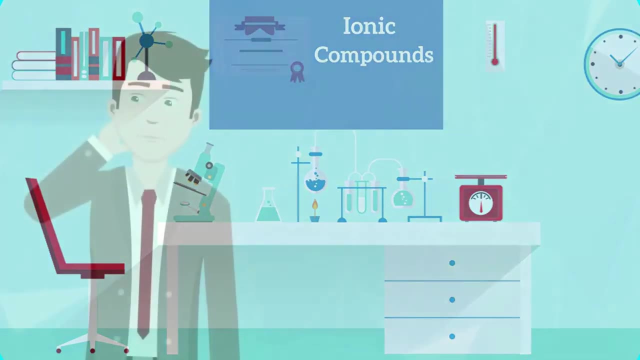 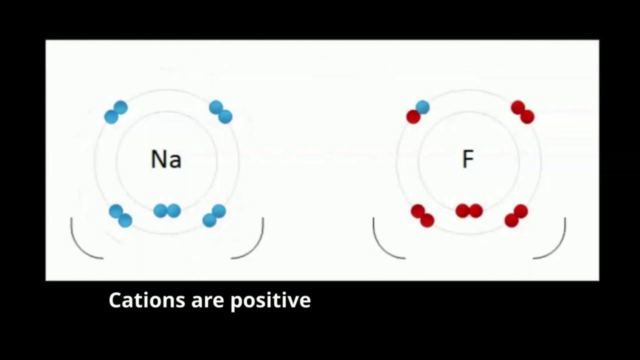 like sugar and others do not like lipids. Starting with our H2O medications, I used a 2 L氼 benut regularly. Most covalent compounds are poor conductors of electricity. Ionic compounds are neutral compounds made up of positively charged ions called cations and negatively charged ions. 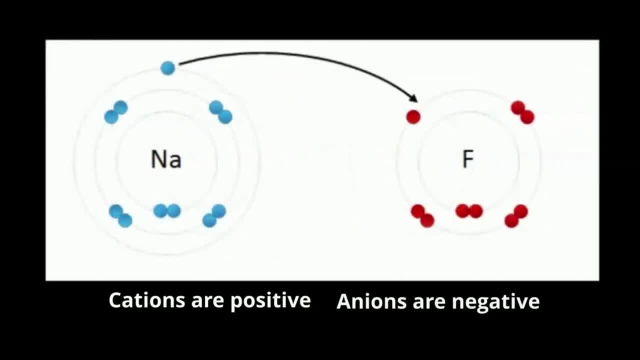 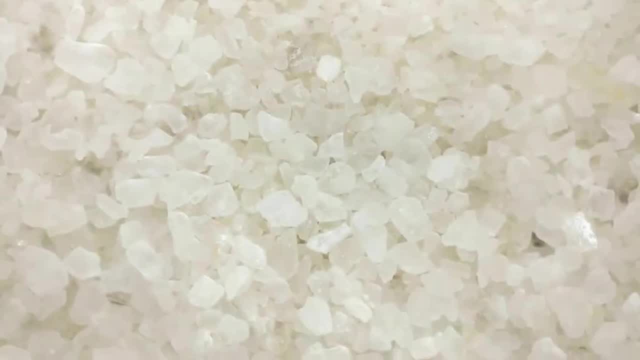 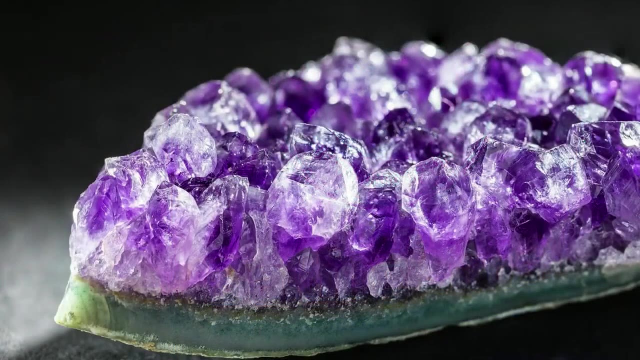 called anions. This results in a very strong bond that holds the compound together. Some common examples include sodium dechloride or table salt, industrium bicarbonate or baking soda and amethyst. 4.. ominine freak of quartz and cinnabar, which is a crystal. Let's take a look at these. 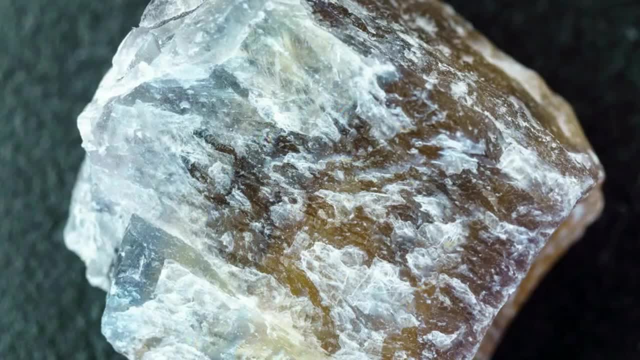 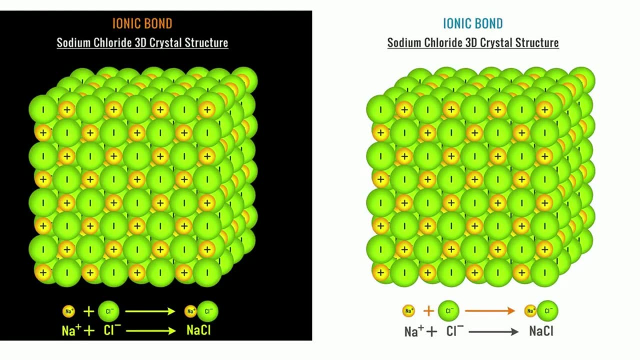 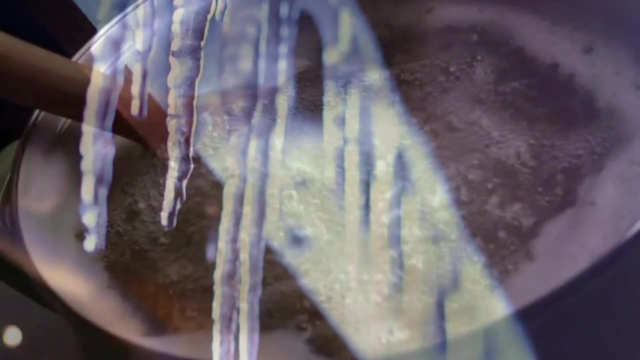 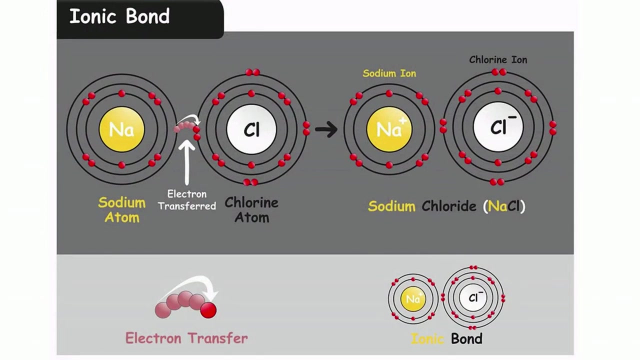 properties. Many ionic compounds are solid crystals at room temperatures. The electrostatic bond creates repeating patterns. that creates crystals. Ionic compounds have high melting and boiling points. The bonds in ionic compounds are very strong and take a lot of energy to break. Ionic compounds are hard and